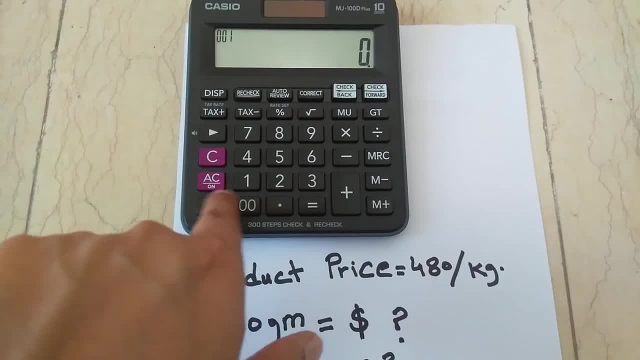 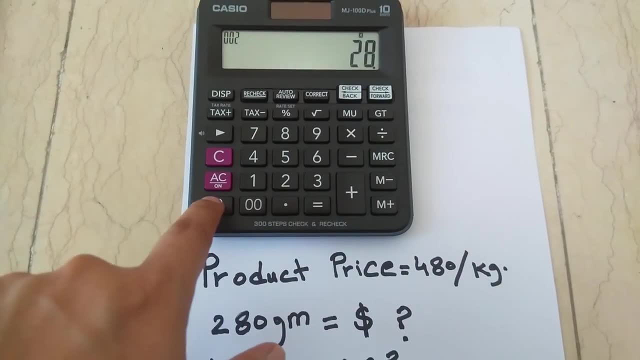 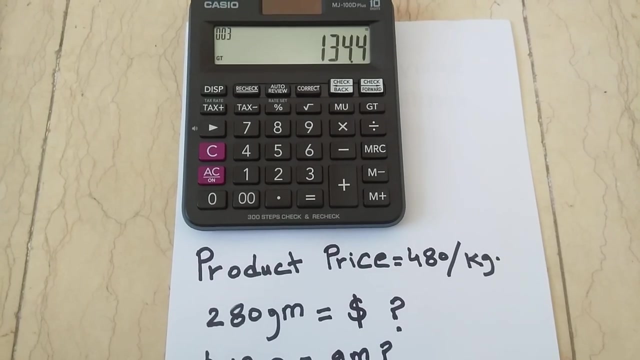 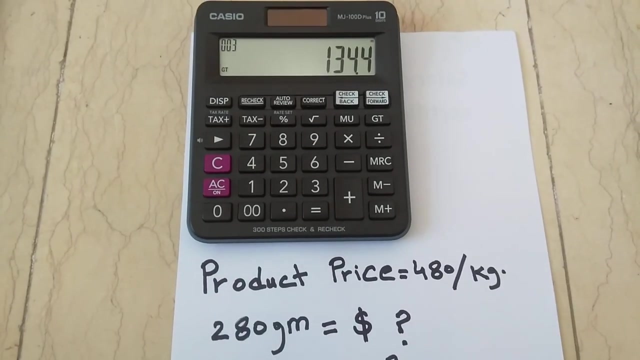 0.48 multiply by 2, sorry, 0.48 multiply by 280. okay, guys, so 134.4 is the answer. guys, so you have to spend 134 dollars to get 280 gram of that particular product. guys, so this is the first. 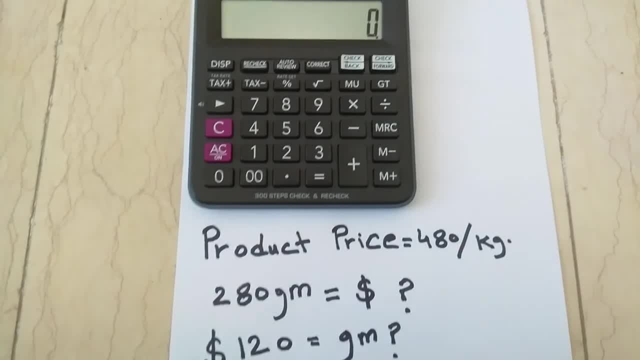 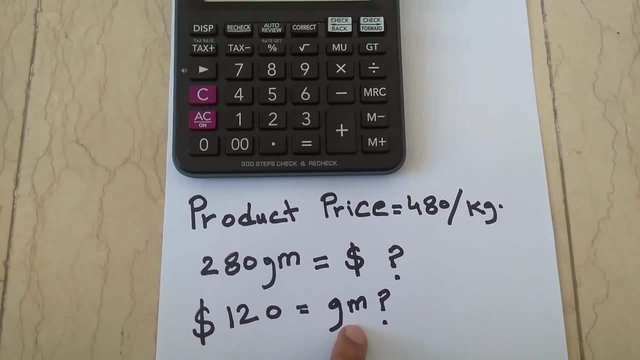 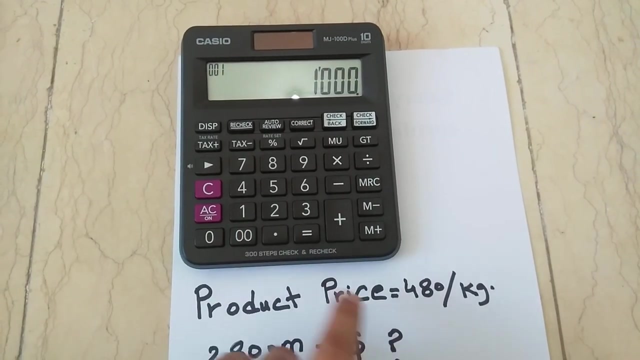 thing, the second thing or the second calculation. for example, you want to spend 120 dollars, guys, and you want to know how much grams you will get. so simply, you have to move to your calculator. you have to type 1000. why i type 1000? because you know 1 kg equal to 1000. 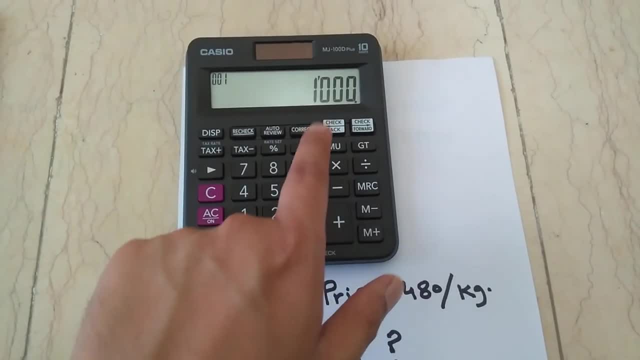 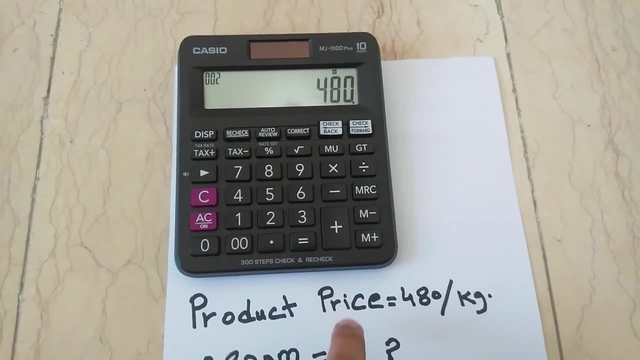 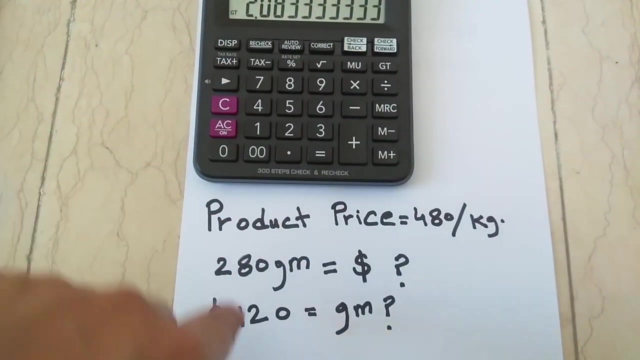 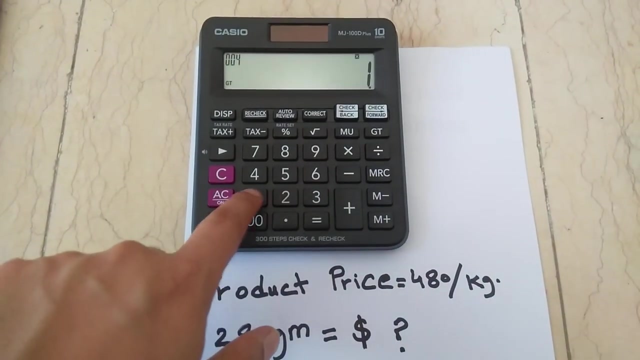 gram. so first you have to type 1000, and then you have to divide it by 480, 480, and then equal. equal to 2.08, guys, okay, guys. so then 2.08 you have to multiply it with 120. so 2.08 multiply by 120. 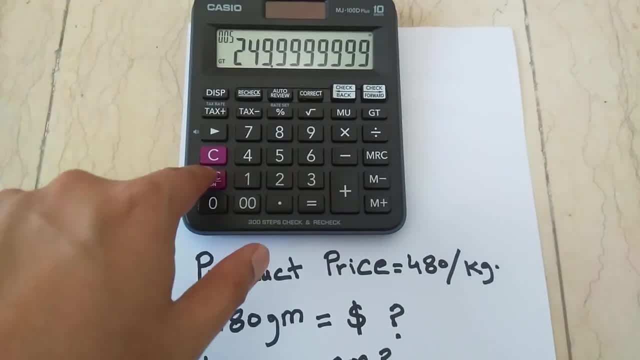 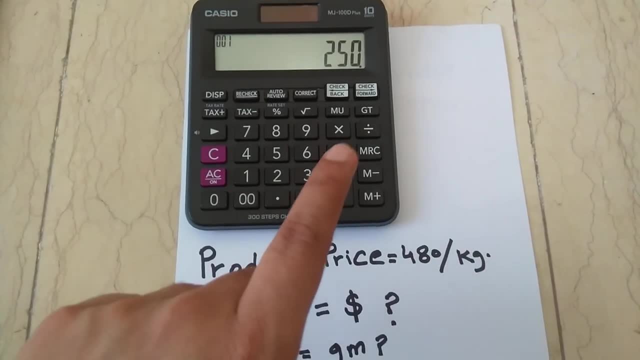 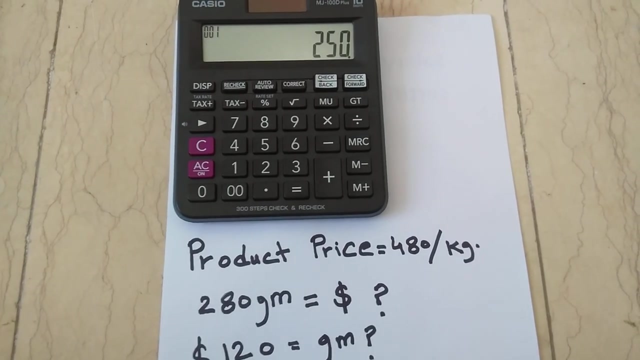 so 249.99, or you can make it 250. so when you spend 120 dollars, you will get 250 gram of that product, guys. so this is how you guys will know the value, or you guys will know the total grams you will get for a certain value, guys. so this is. 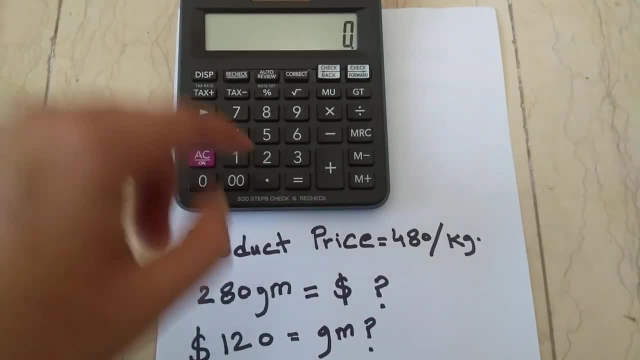 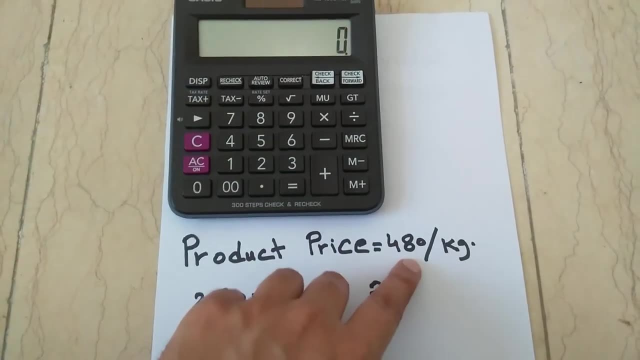 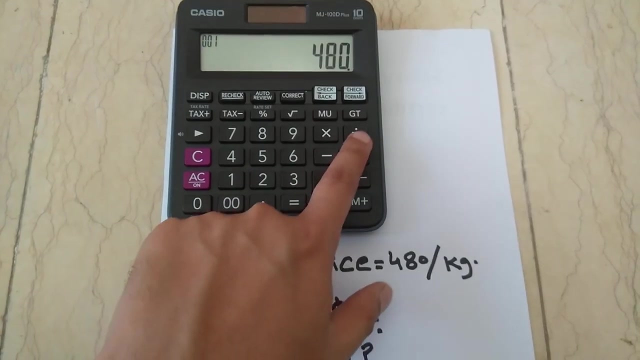 very simple technique, guys. simply, you have to follow two steps. in the first step, if you want to know how much dollars you have to spend for certain gram, simply you have to divide the total value of the product divided with 1000. 480 divided by 1000- okay, this is the answer. then multiply this. 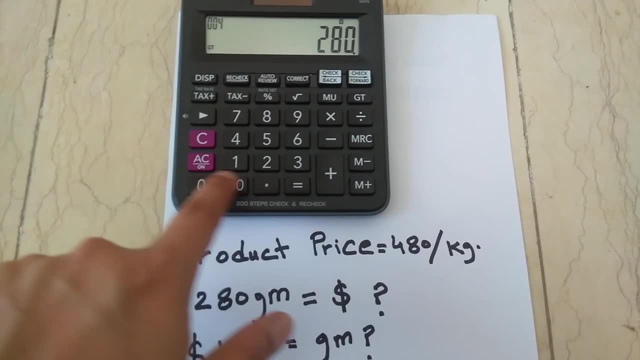 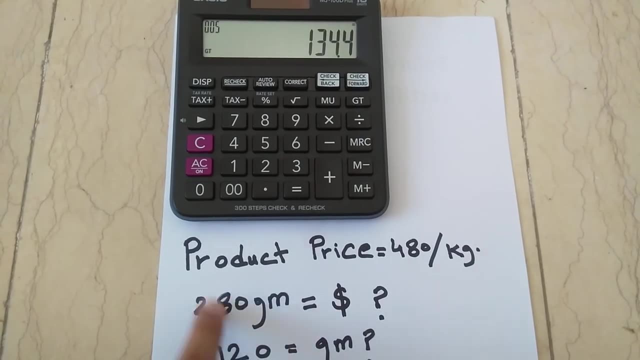 480 by .48 with 280 grams. so multiply 280, so 134 is the answer. so you have to spend 134 dollars to get to 280 grams, guys, okay. so the second thing which i explained to you: you, if you want to spend 120 and you want to,